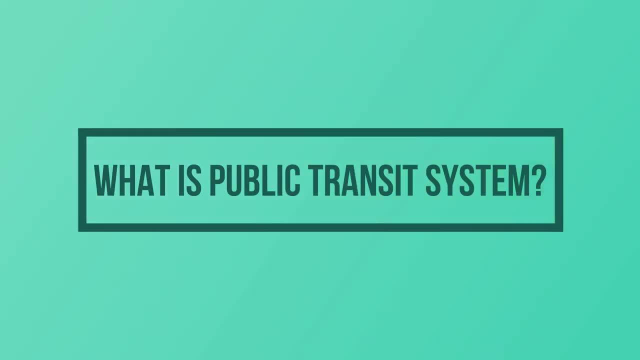 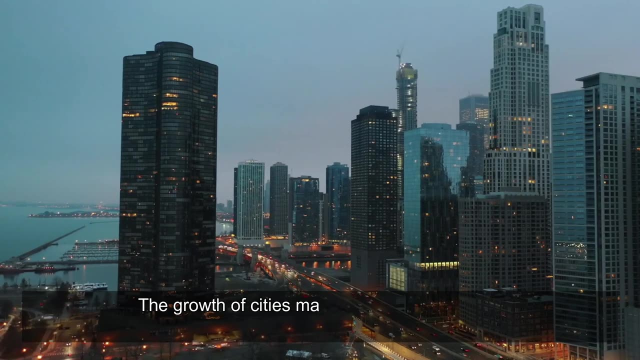 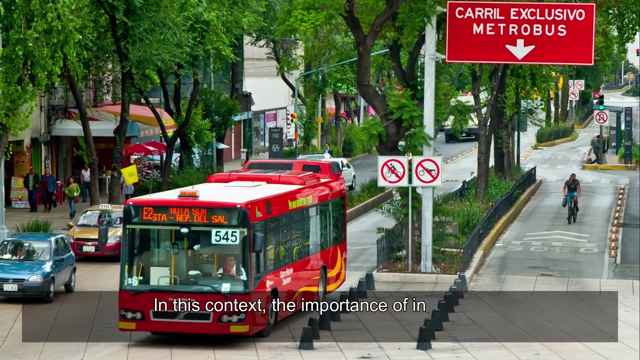 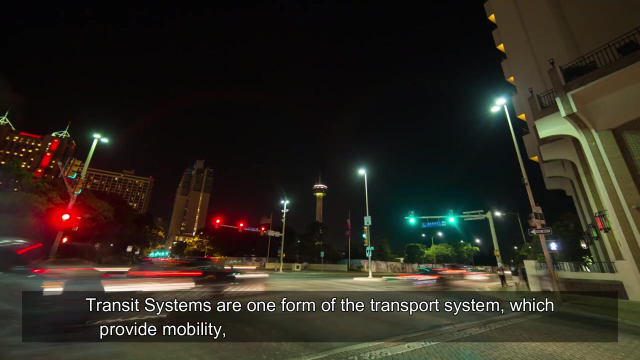 What is public transit system? Cities play a vivacious role in helping economic development and prosperity. The growth of cities mainly depends upon their social, physical, social and established infrastructure. In this context, the importance of intra-urban and inter-urban transportation is paramount. Transit systems are one form of the transport system which provide 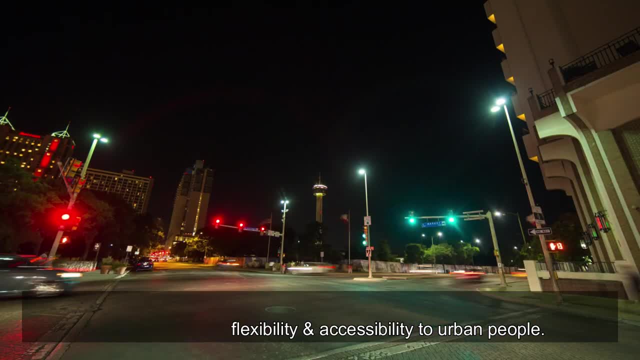 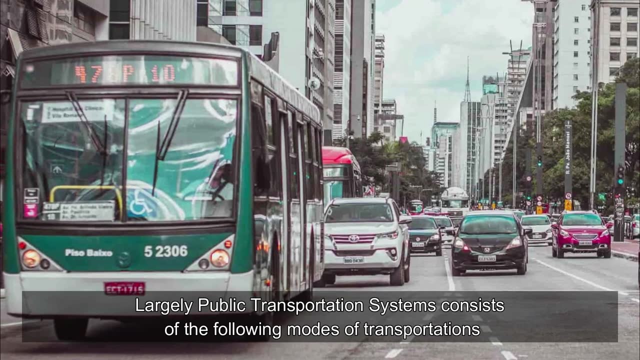 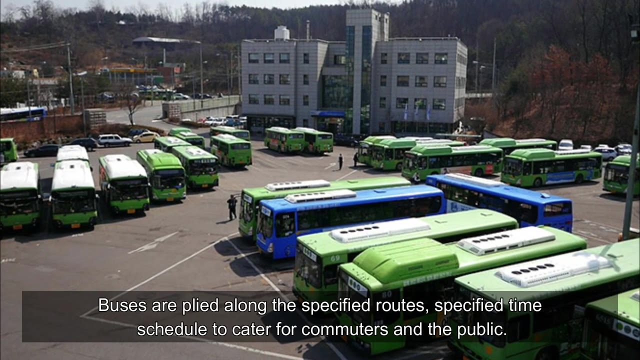 mobility, flexibility and accessibility to urban people. What are the types of public transit system? Largely, public transportation systems consists of the following modes of transportations: Bus: Buses are plied along the specified routes, specified time schedule, to cater for commuters. 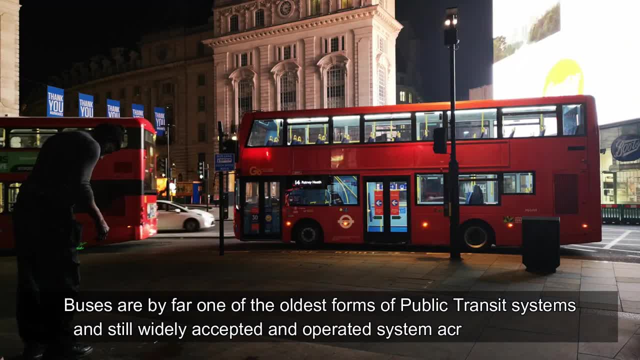 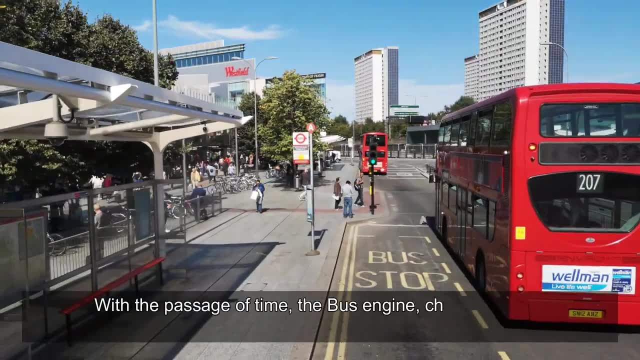 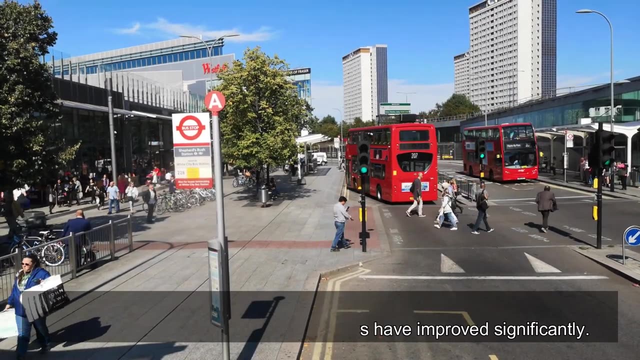 and the public. Buses are by far one of the oldest forms of public transit systems and still widely accepted and operated system across the globe. With the passage of time, the bus engine, chassis, seats, routes and other operational parameters have improved significantly. Now the journey through buses are more predictable, comfortable. 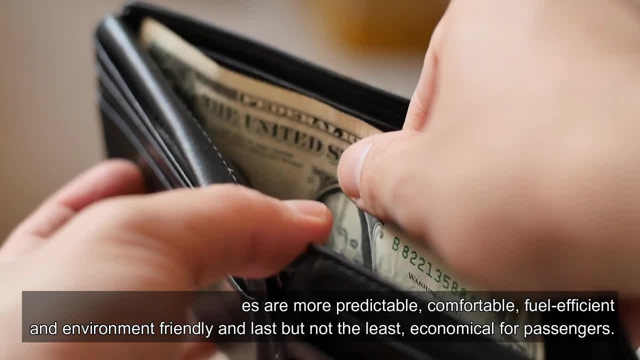 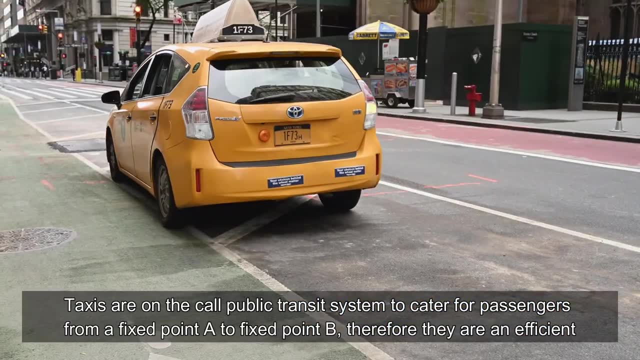 fuel-efficient and environment-friendly and, last but not the least, economical for passengers. Taxis- Taxis are on the call public transit system to cater for passengers from a fixed point A to fixed point B. therefore they are an efficient, comfortable on-demand system. but 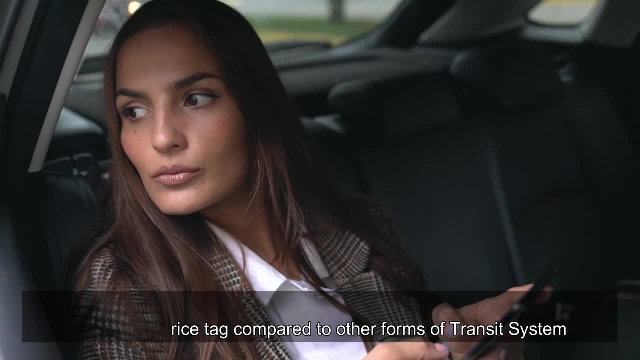 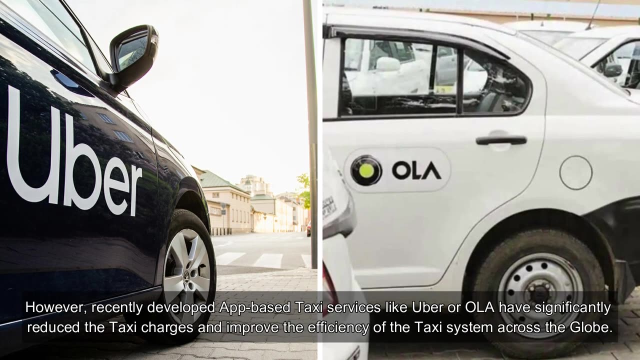 comes with an expensive cost. Taxis are on the call public transit system to cater for passengers with a higher price tag compared to other forms of transit system. However, recently developed app-based taxi services like Uber or Ola have significantly reduced the taxi charges and. 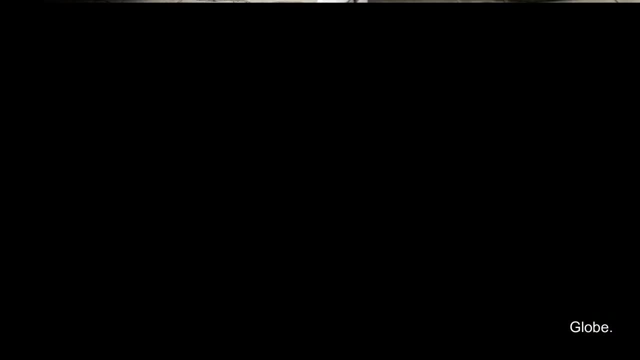 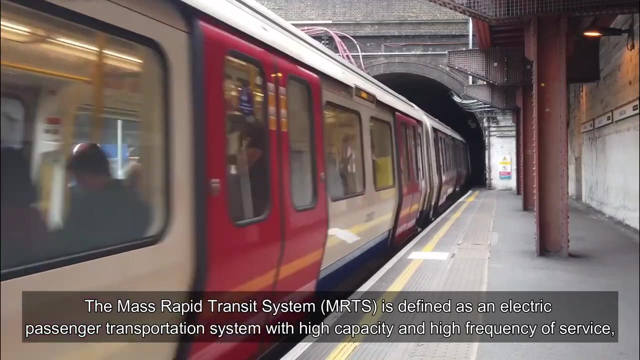 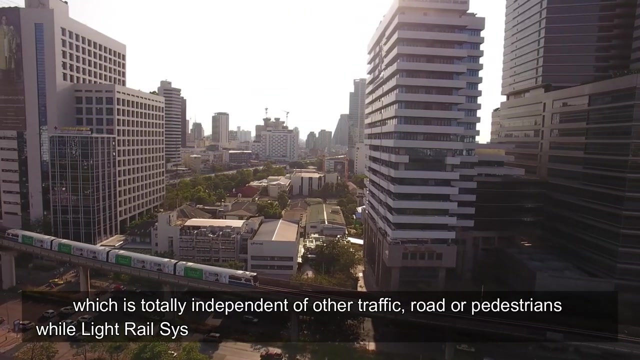 improved the efficiency of the taxi system across the globe. Mass rapid transit and light rail systems. The mass rapid transit system is defined as an electric passenger transportation system with high capacity and high frequency of service which is totally independent of other traffic, road or pedestrian service. 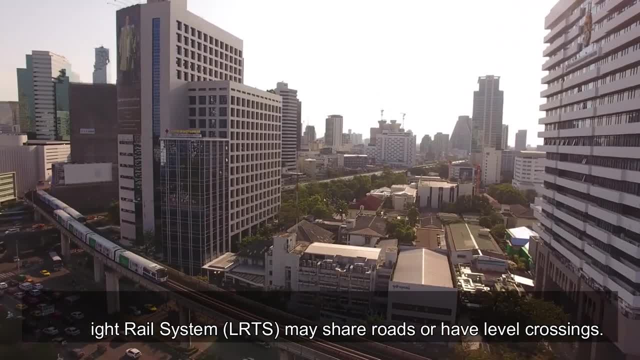 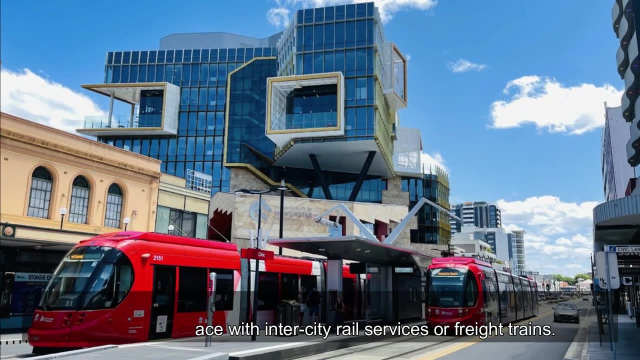 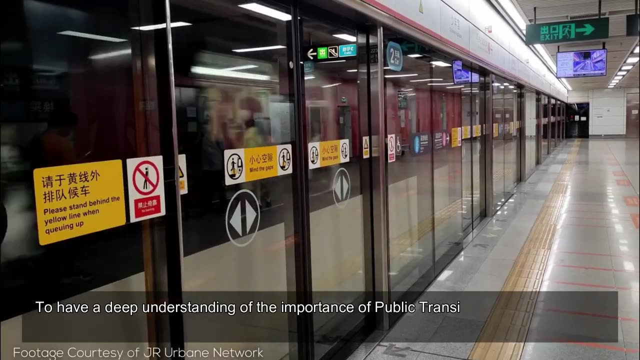 while light rail system, LRTS, may share roads or have level crossings. Additionally, these transit systems do not share their space with intercity rail services or freight trains. What are the advantages and disadvantages of public transit system? To have a deep understanding of the 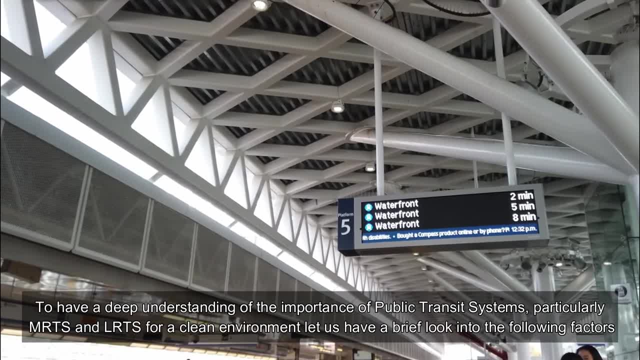 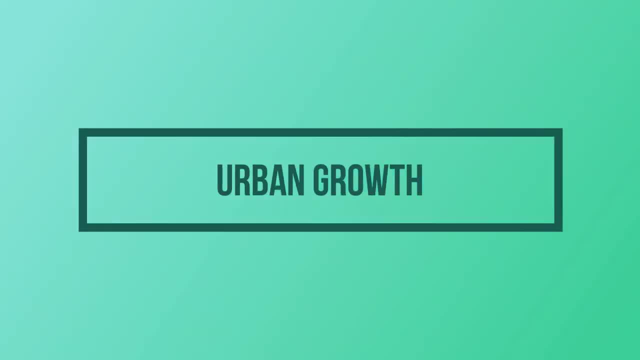 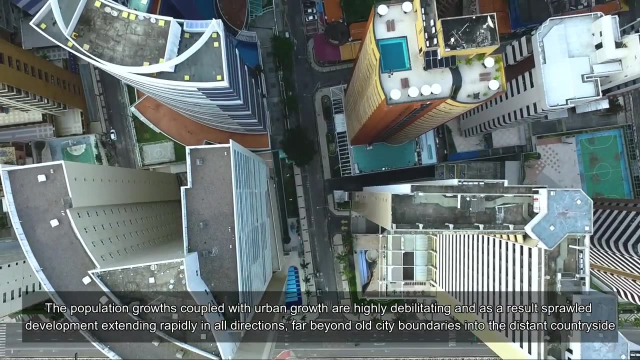 importance of public transit systems, particularly MRTS and LRTS, for a clean environment. let us have a brief look into the following factors: Urban growth: The population growths coupled with urban growth are highly debilitating and, as a result, sprawl development extending rapidly in. 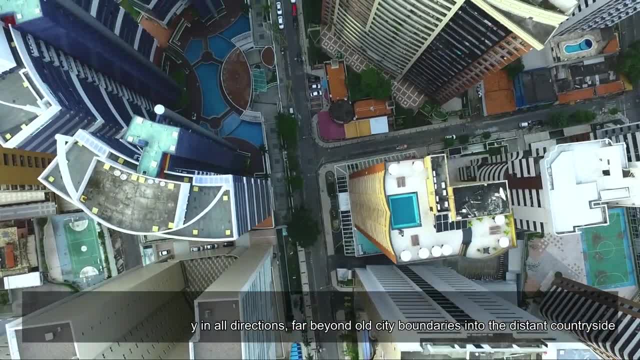 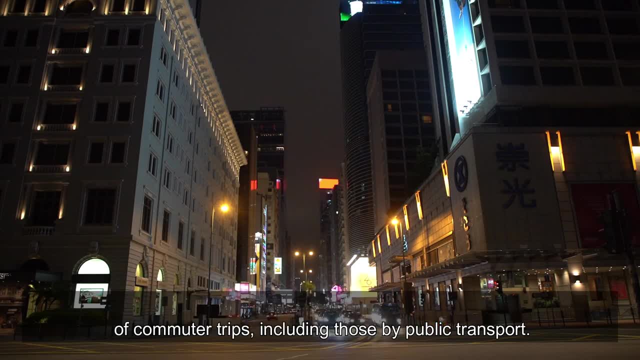 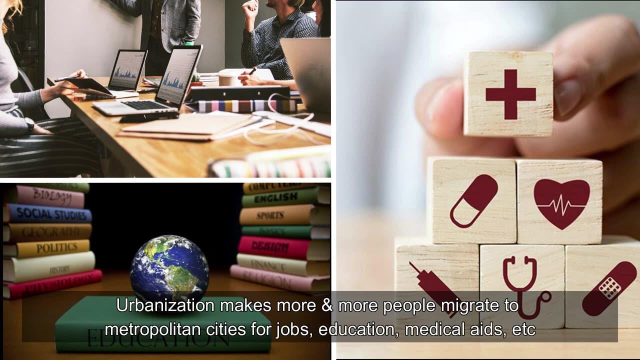 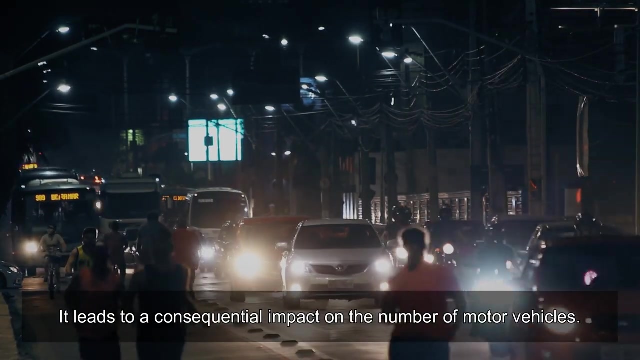 all directions, far beyond old city boundaries into the distant countryside. That also has greatly increased the number and length of commuter trips, including those by public transport. Vehicular growth, Urbanization makes more and more people migrate to metropolitan cities for jobs, education, medical aids, etc. It leads to a consequential impact on the number of motor. 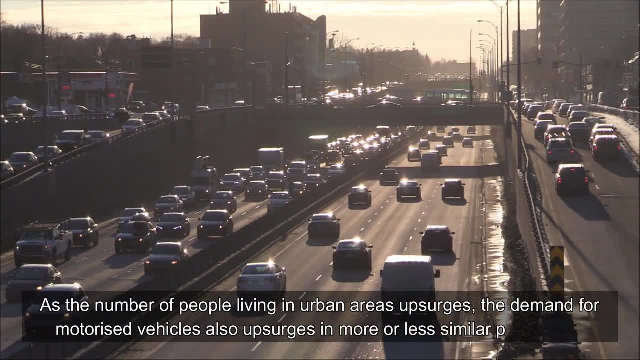 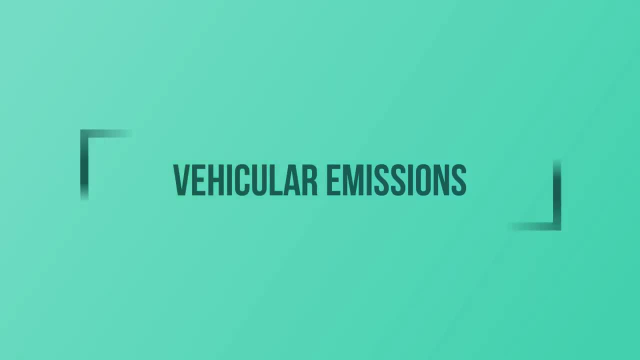 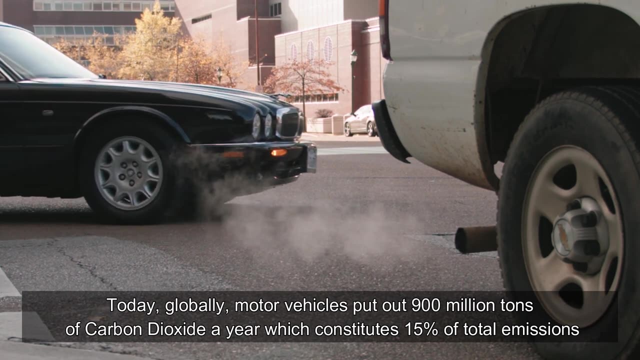 vehicles. As the number of people living in urban areas upsurges, the demand for motorized vehicles also upsurges, in more or less similar proportions, Vehicular emissions. Today, globally, motor vehicles put out 900 million tons of carbon dioxide a year, which constitutes 15% of total. 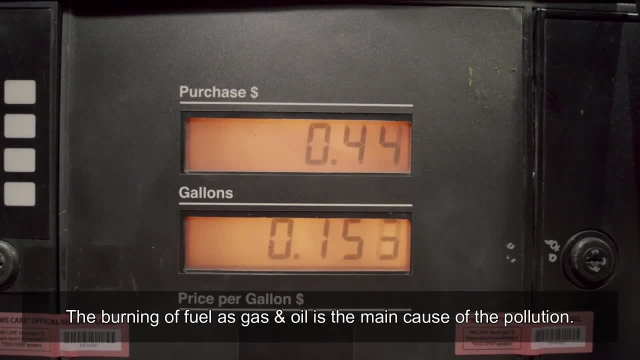 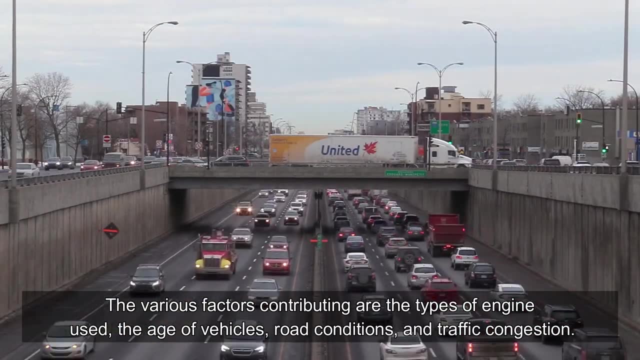 emissions. The burning of fuel and gas is a major factor in the growth of urbanization. Oil, as gas in oil, is the main cause of the pollution. The various factors contributing are the types of engine used, the age of vehicles, road conditions and traffic congestion. 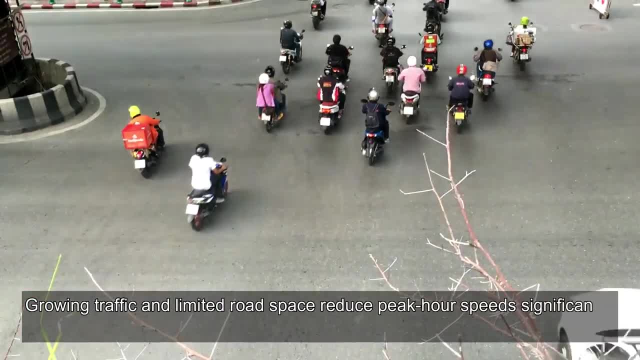 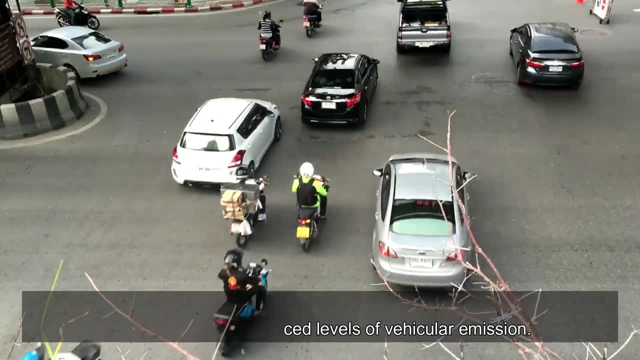 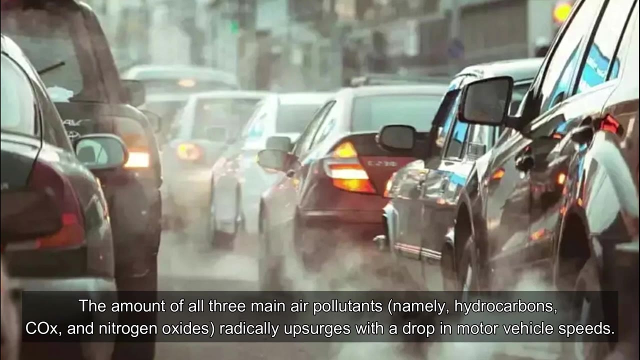 Traffic congestion, Growing traffic and limited road space reduce peak hour speeds significantly. This also implies advanced levels of vehicular emission. The amount of all three main air pollutants, namely hydrocarbons, COX and nitrogen oxides, radically upsurges. 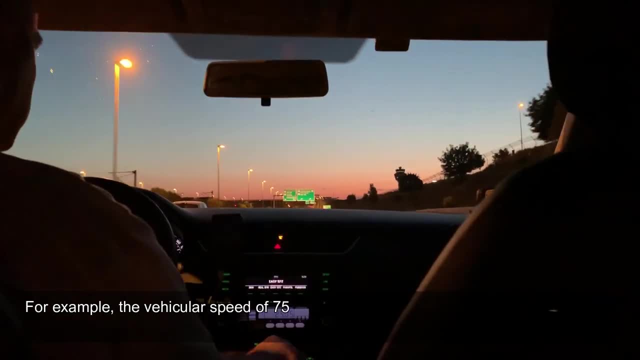 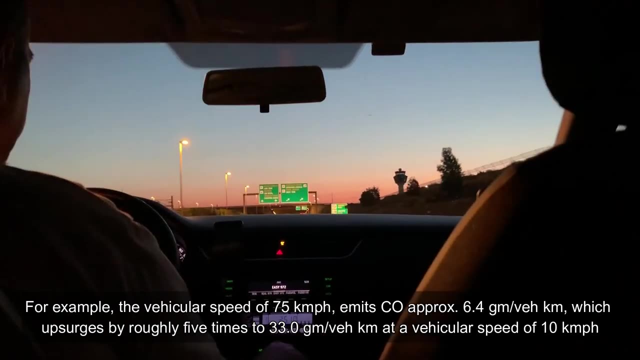 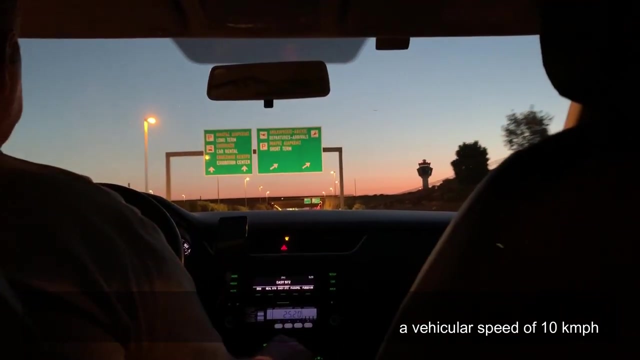 For example, the vehicular speed of 75 km per hour emits CO-approximate 6.4 gm-slash-ve km, which upsurges by roughly 5 times to 33.0 gm-slash-ve km at a vehicular speed of 10 km per hour. 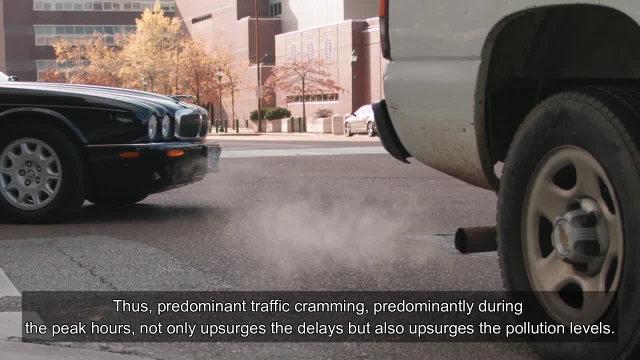 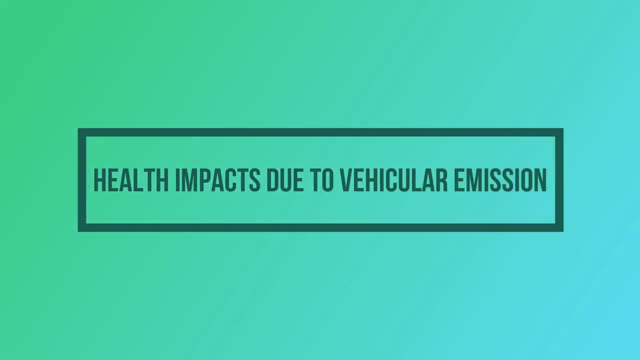 Thus, predominant traffic cramming, predominantly during the peak hours, not only upsurges the delays, but also upsurges the pollution levels. Health impacts due to vehicular emission. The major air pollutants due to vehicular emissions severely affect human health. 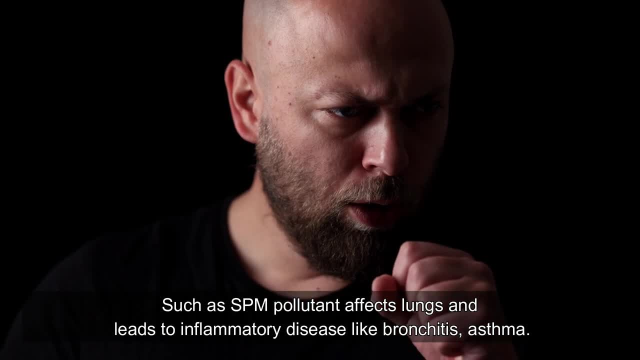 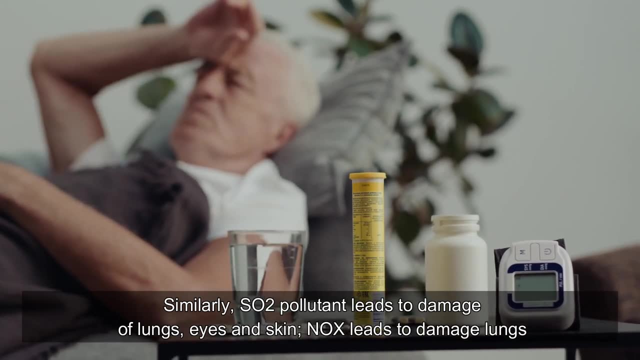 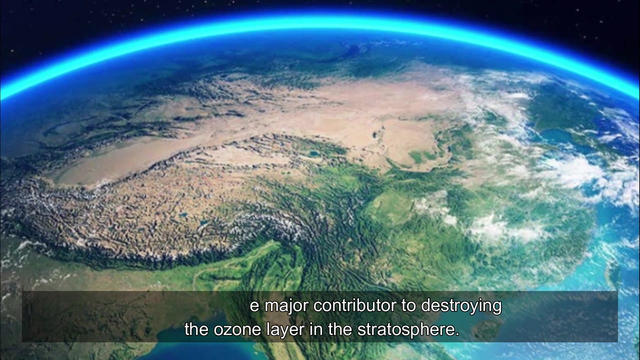 Such as SPM. pollutant affects lungs and leads to inflammatory disease like bronchitis, asthma. Similarly, SO2 pollutant leads to damage of lungs, eyes and skin. NOx leads to damage lungs. NOx is also the major contributor to destroying the ozone layer in the stratosphere.